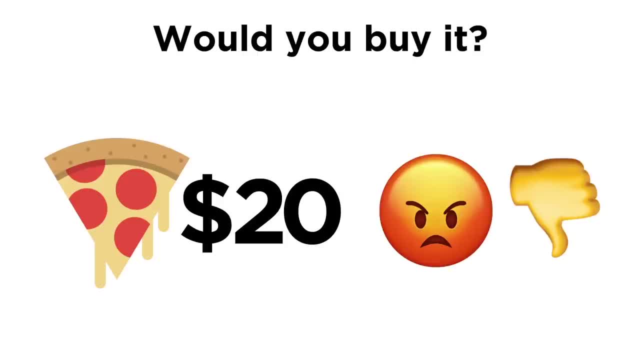 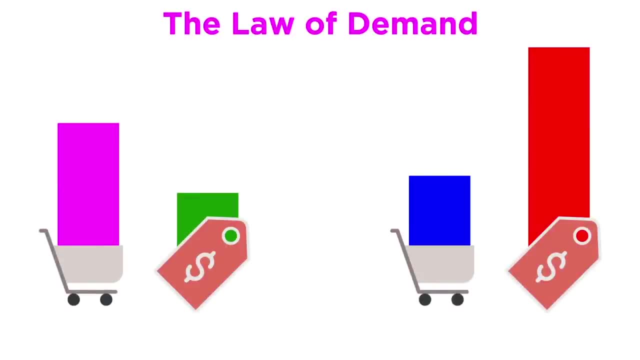 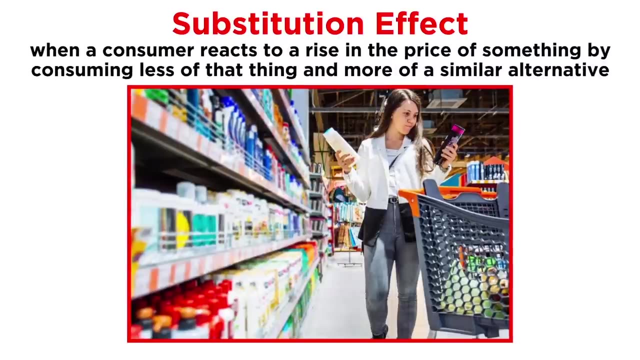 Perhaps we would buy it only if we were starving and knew that there would be no other opportunity to buy food for a long time. Now, there are many variables which can influence demand. One such variable is known as the substitution effect, which takes place when a consumer reacts. 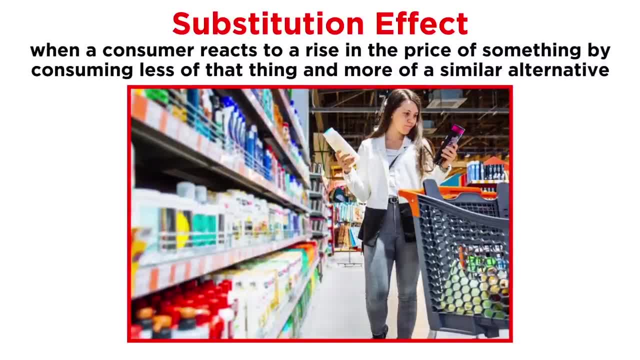 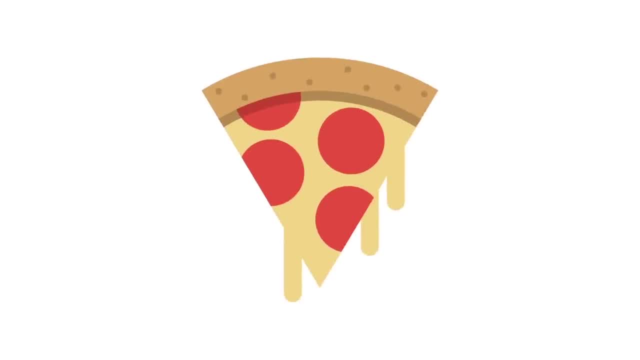 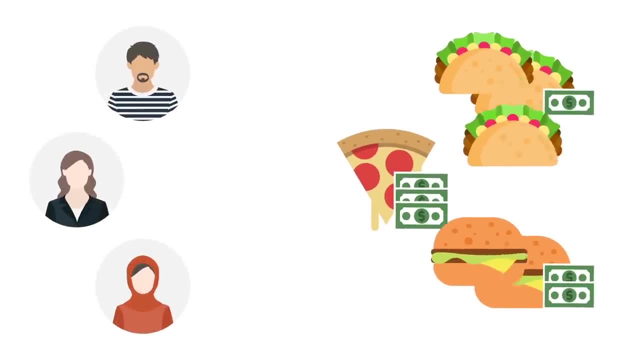 to a rise in the price of something by consuming less of that thing and more of that thing. For example, when the price of pizza becomes more expensive compared with other foods, consumers become more likely to buy a substitute food item like tacos or hamburgers. 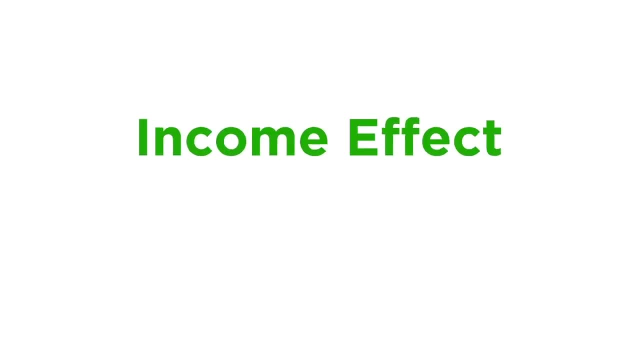 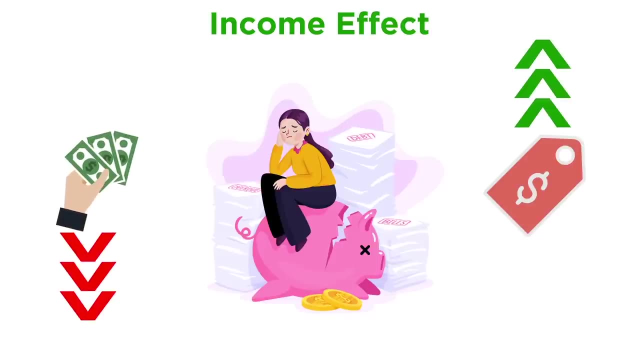 Another such variable is the income effect. Rising prices make us all feel more poor. When prices rise, we cut back on what we buy if our income does not go up. When you buy less of something, you can buy less of it. When you buy less of something, you can buy less of it. 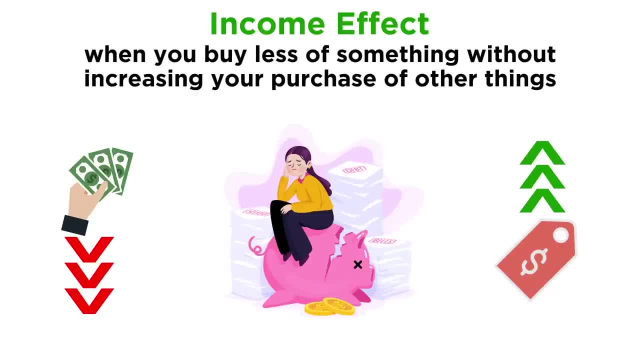 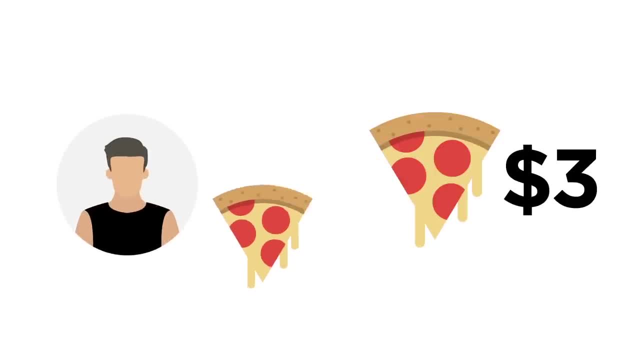 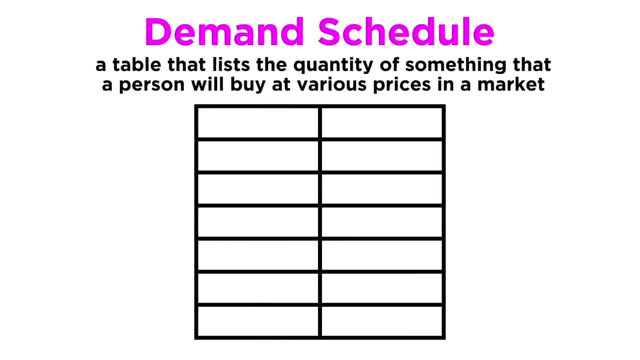 Without increasing your purchase of other things. that is the income effect. So if the price of a slice of pizza goes from two dollars to three dollars, you might buy only three slices instead of four. We can illustrate this in a demand schedule, which is a table that lists the 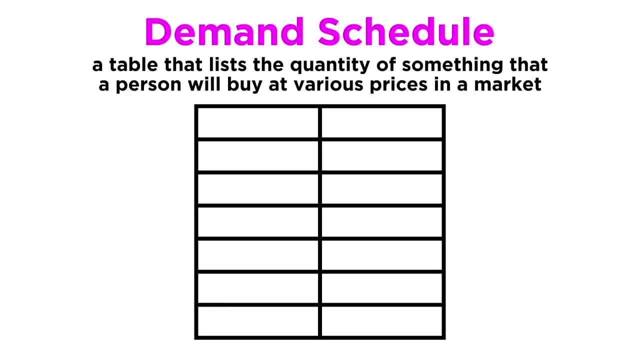 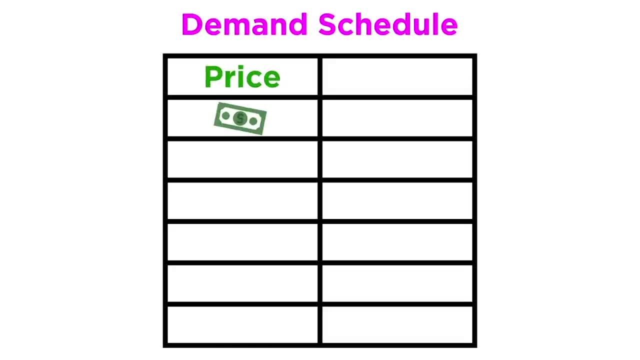 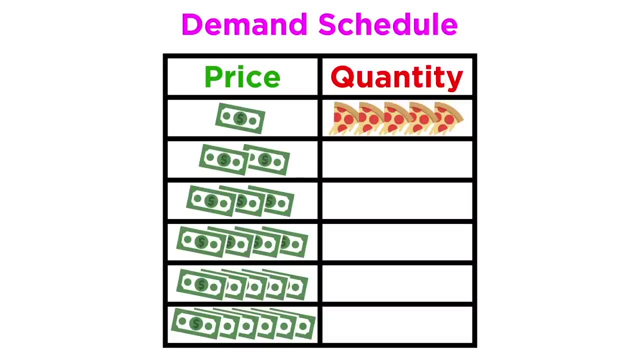 quantity of something that a person will buy at various prices in a market. Sticking with the pizza example, in the first column we have the price of a slice of pizza from one dollar all the way to six, And in the second column we have the quantity demanded, which might be five slices when they 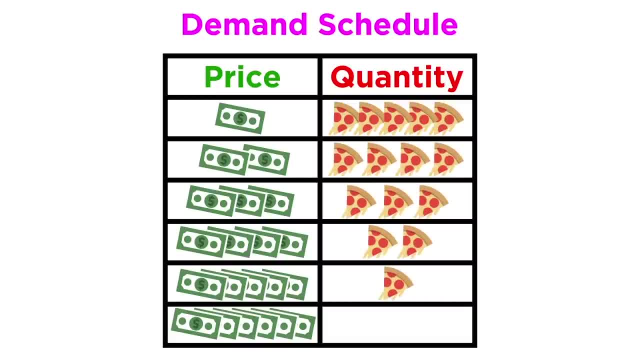 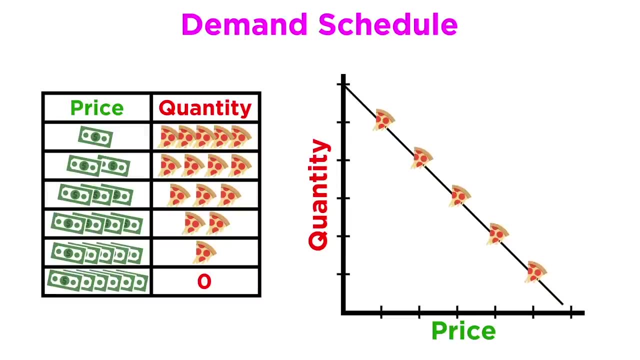 are only a buck and decreasing by one for every dollar increase in slices, in the limit of six dollars per slice where it is deemed by the consumer to be too expensive to purchase. Now what if we plotted these numbers on a graph? The result would be a downward-sloping demand. 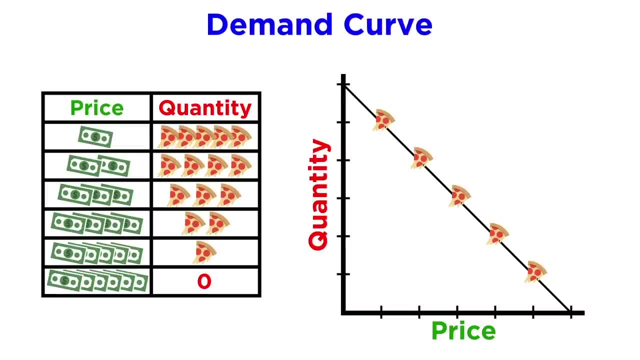 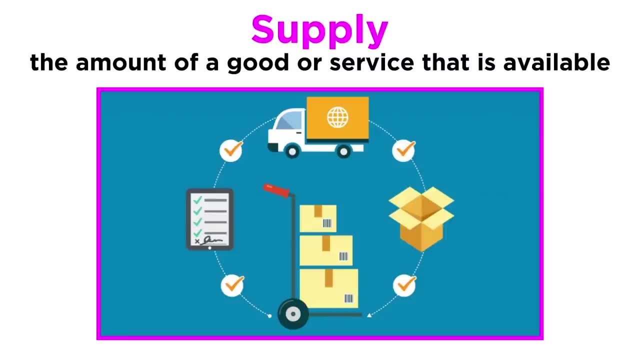 graph, also commonly called a demand curve. This is just a graphical representation of a demand schedule and can be a more useful way of visualizing this data. Okay, with demand covered, now let's look at supply. Supply is the amount of a good or service. 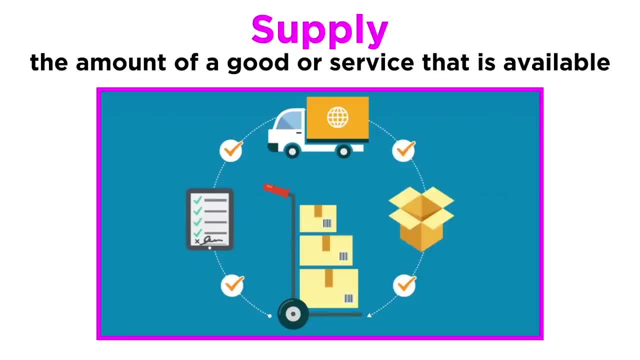 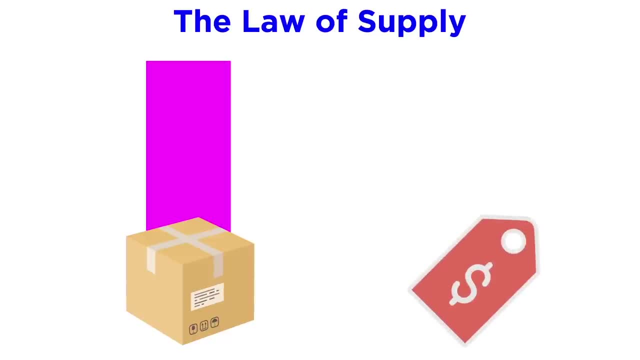 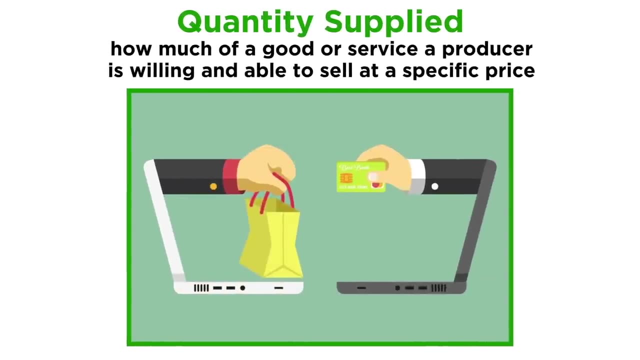 that is available. So how do producers know how much to supply? Well, according to the law of supply, producers offer more of a good or service as its price increases and less as its price falls. Economists use the term quantity supplied. 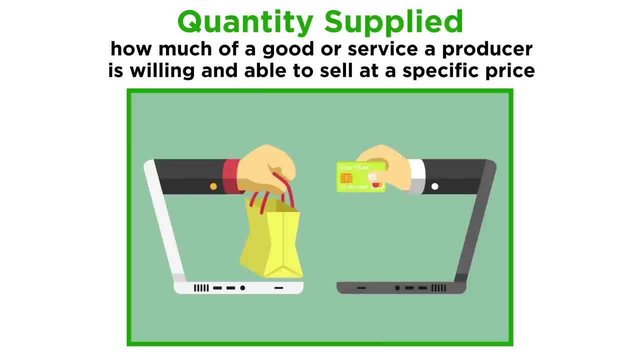 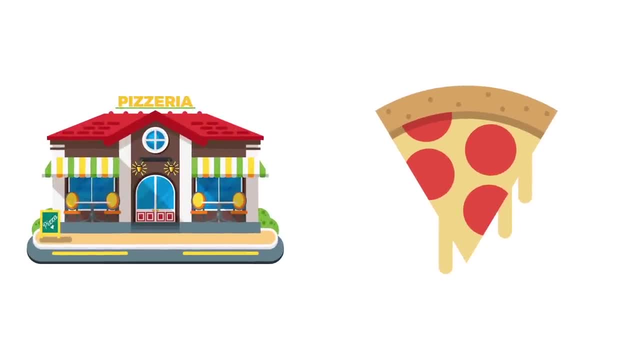 to illustrate how much of a good or service a producer is willing and able to sell at a specific price. Let's stick with pizza, for our example. If the pizza shop is already making money selling lots of slices of pizza all day, the promise of higher revenues generated by each sale. 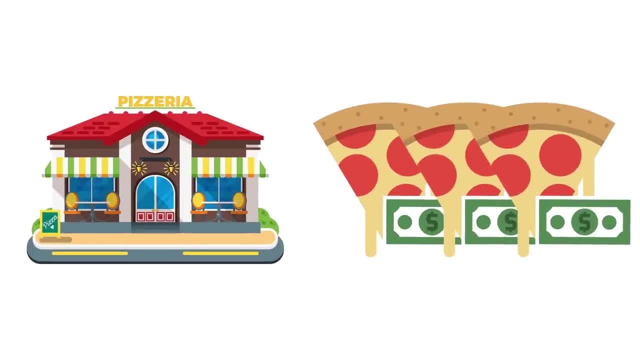 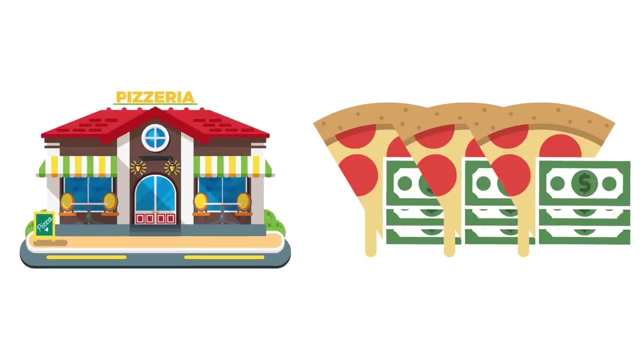 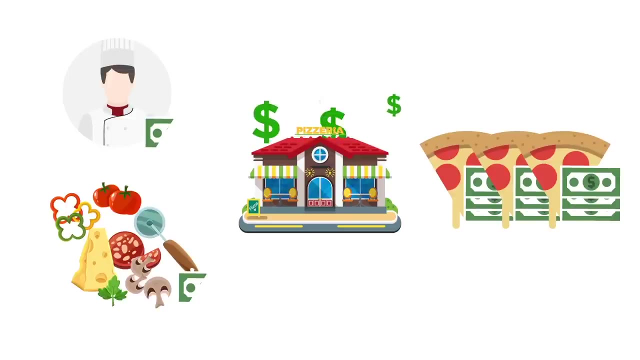 motivates the pizza shop to make more pizza, Assuming that the price of pizza were to be set by some outside figure. if the price of pizza rises but the pizza shop's cost of making pizza stays the same, the pizza shop will earn a higher profit on each slice. The owner of the 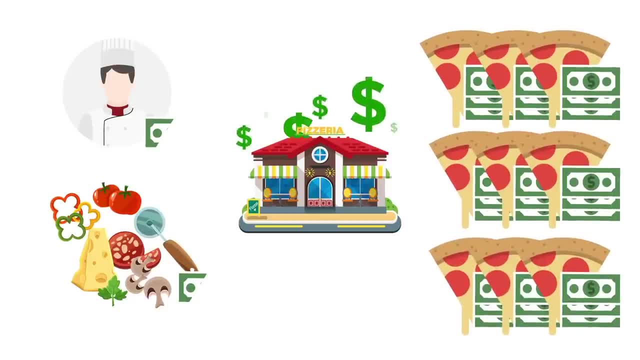 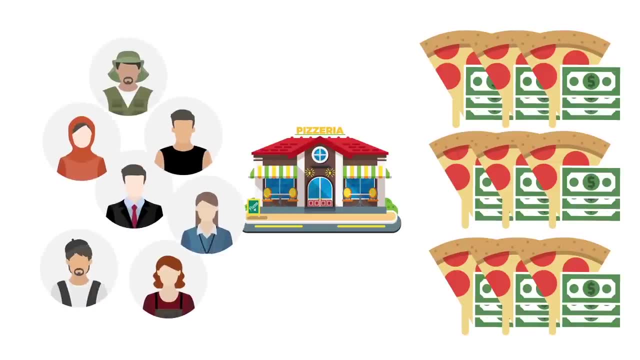 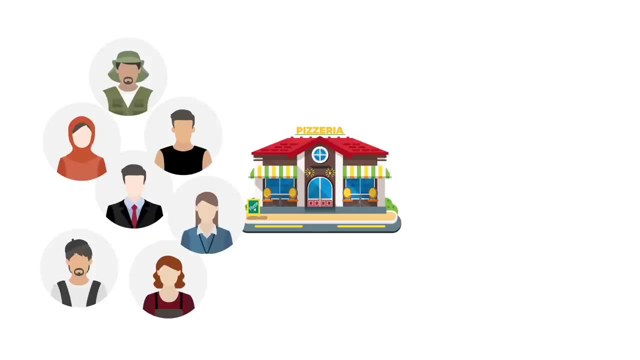 pizza shop understands that making more pizza makes sense in order to take advantage of the higher prices. Now perhaps the demand is so high that the pizza shop can't even keep up with the necessary supply. Customers show up and by noon there is no more pizza. This may lead to a change. 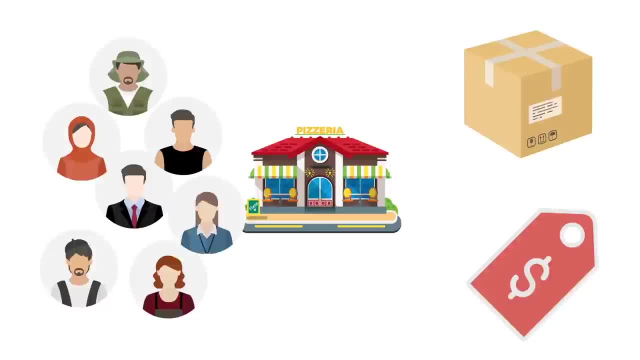 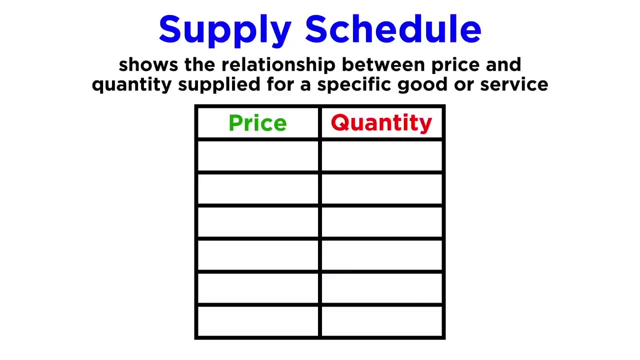 in either the price or the supply. Similar to a demand schedule, supply schedule shows the relationship between price and quantity supplied for a specific good or service, or how much of a good or service a supplier will offer at various prices. Like a demand schedule, a supply schedule lists supply for a very specific set of conditions, For example, 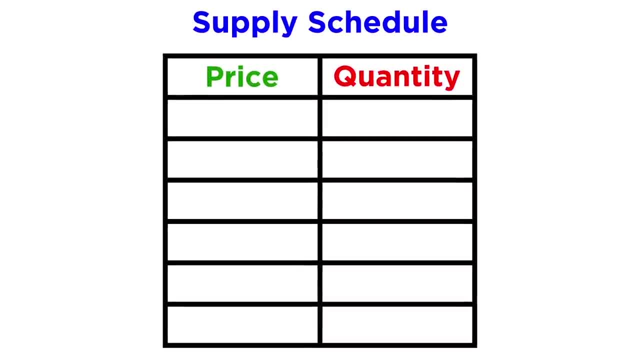 let's list the price of the pizza in the first column, again from $1 to $6.. Then, in the second column, let's list the slices that will be sold at a certain price. For example, let's list the slices that will be supplied per day, starting with 100 and going up by 50 for each dollar increase. 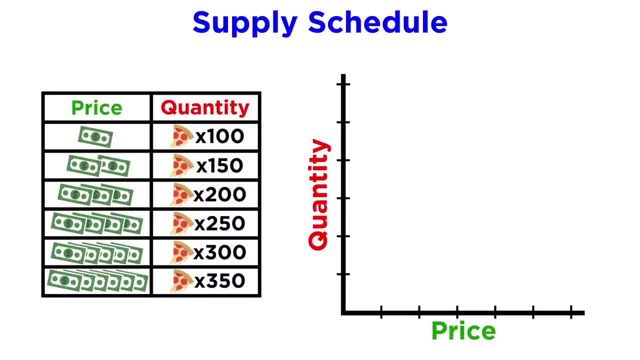 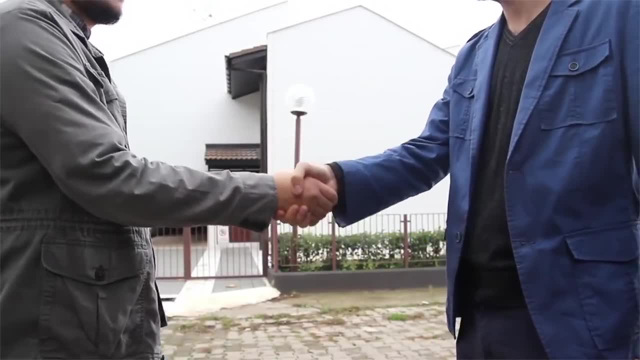 in price. Again, we could plot these numbers on a graph and the result would be an upward-sloping supply graph, commonly called a supply curve. This is a graphical representation of a supply schedule. When buyers and sellers come together in a market, supply and demand have a close relationship. 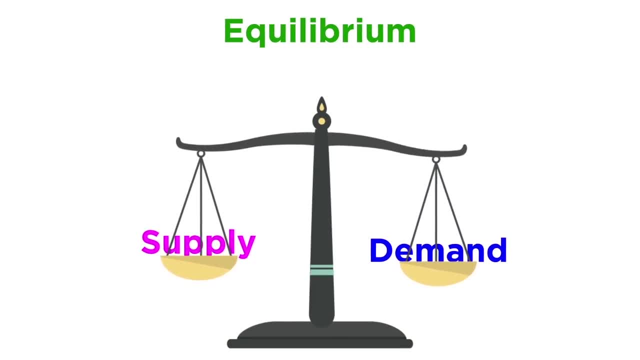 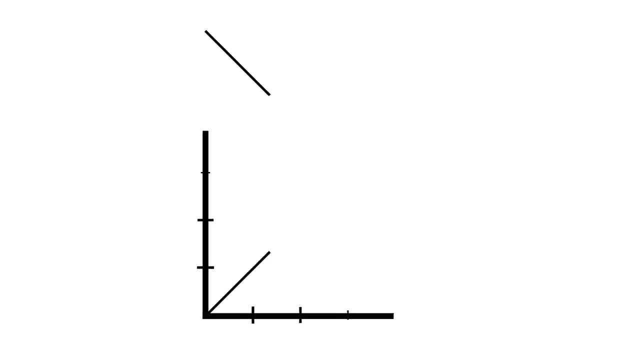 Supply and demand create an equilibrium in the market. supply and demand create an equilibrium in the market. supply and demand create an equilibrium in the market, which is the point of balance at which the quantity demanded equals the quantity supplied. If we draw the demand and supply curves on the same plot, we can identify the point where the